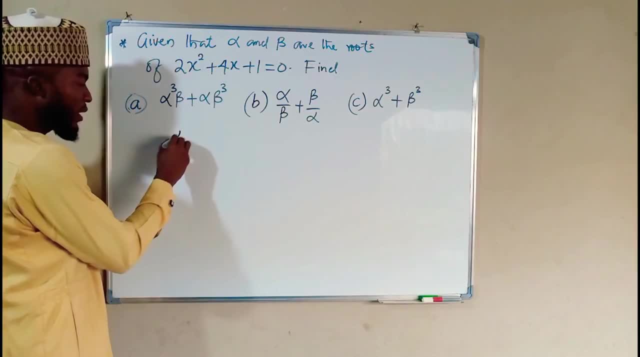 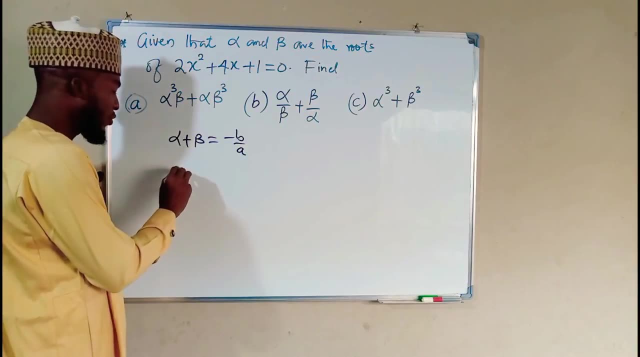 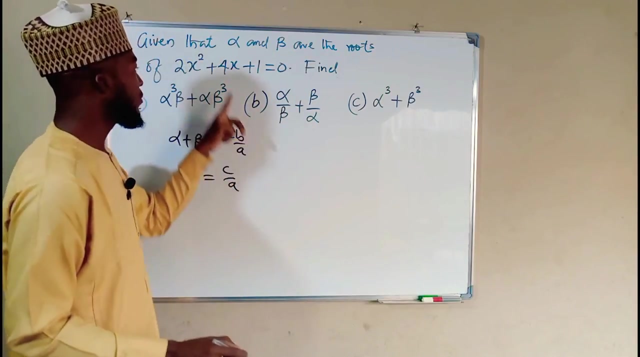 the sum and the product of the quadratic roots. Sum meaning alpha plus beta, which is given as negative, b over a, and the product is alpha times beta, which is given as c over a, and b is the coefficient of the middle term, which we have here as 4.. So we are going to take negative 4. 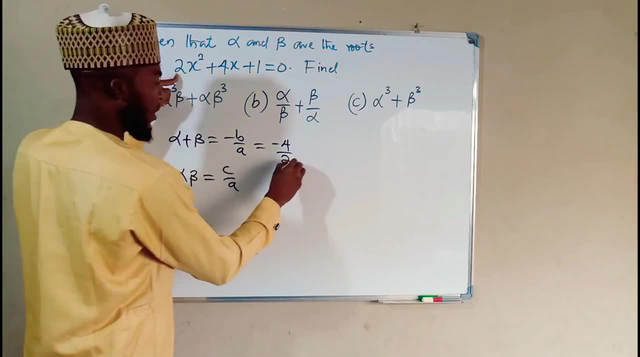 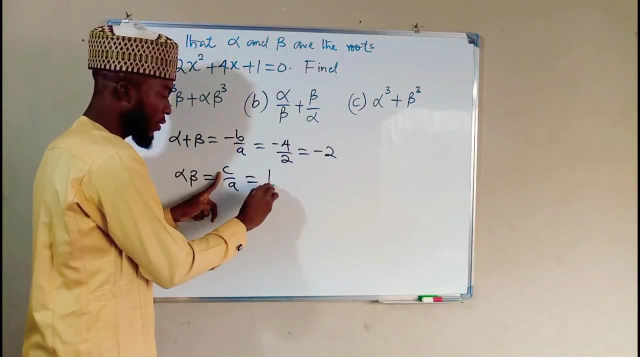 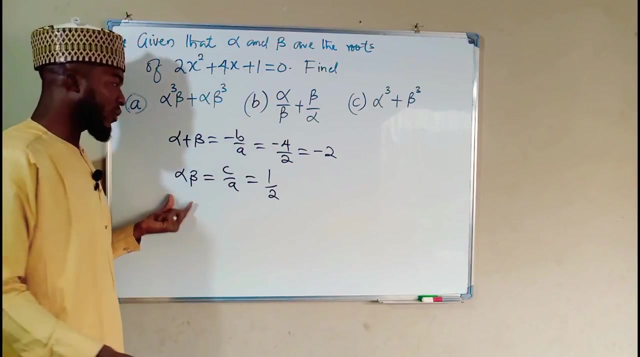 divided by a, and a is the leading coefficient, which is 2.. This is equal to negative 2.. Then for this we have c, which is constant 1 over a, and a is the leading coefficient, which is 2.. Hence we can see that the sum and the product of this quadratic roots 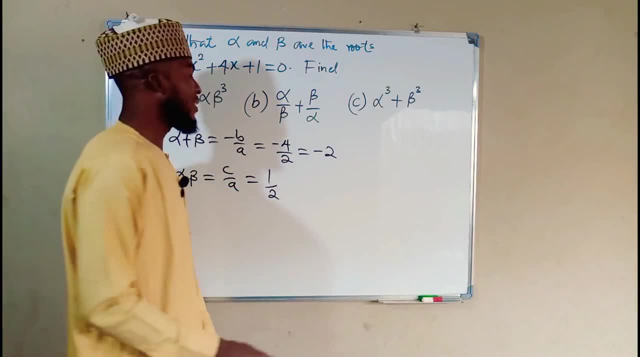 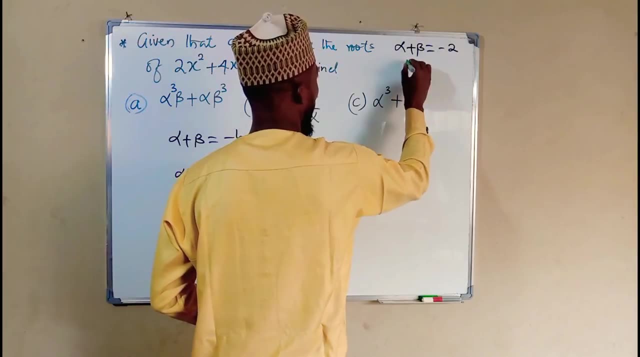 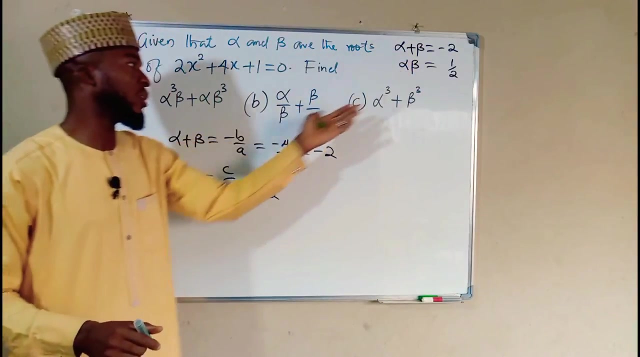 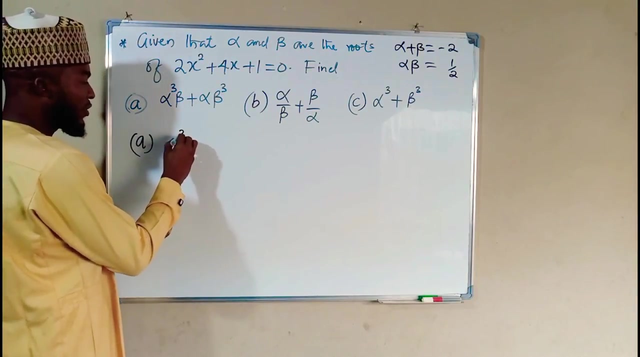 are negative 2 and 1 over 2 respectively, So we can write them aside. Alpha plus beta equals negative 2.. Alpha times beta equals 1 over 2.. Now let us use this information to find the solution for these three problems. The first one: alpha cubed, beta plus alpha beta cubed. 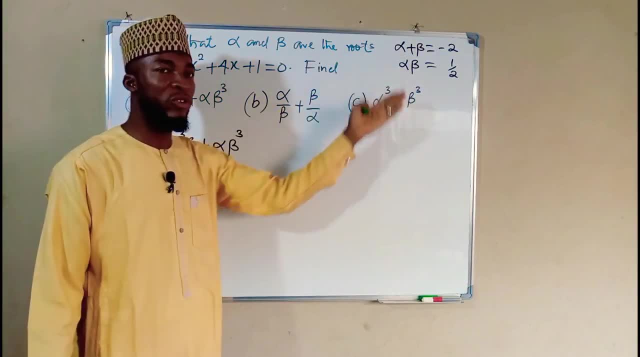 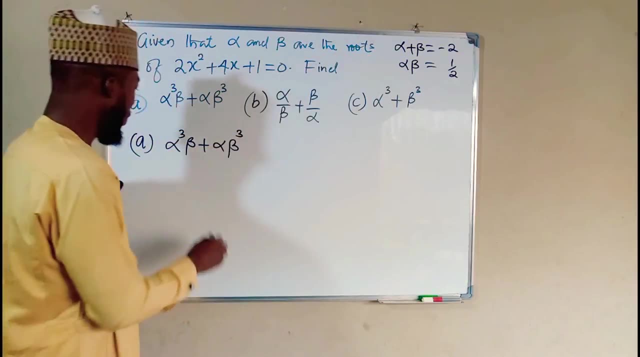 Remember, we do not have anything in this form. All we have is sum and the product. Therefore, let us transform this function in such a way it will contain one of these or all of them. So let's factor out alpha beta so we can see this is the same thing as alpha beta. 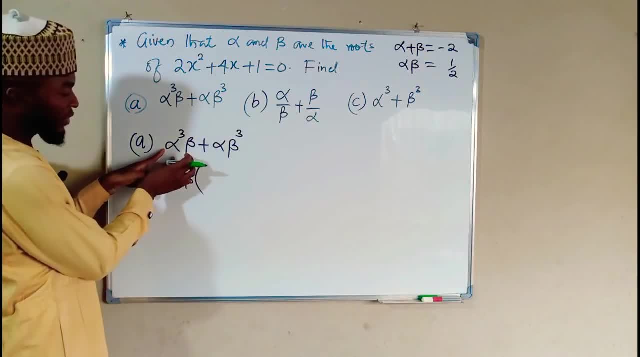 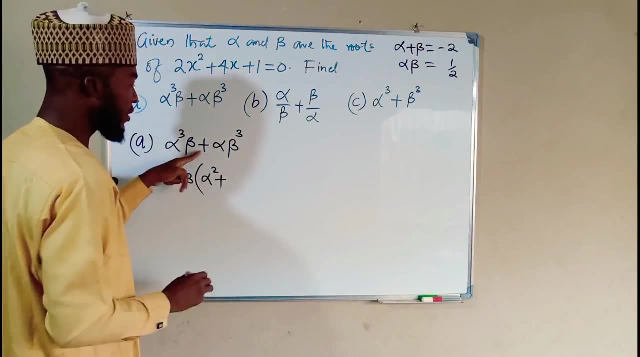 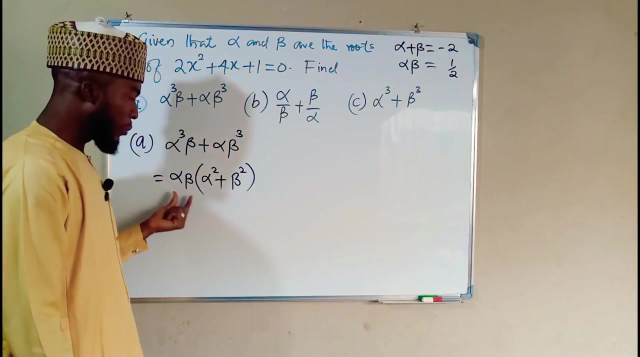 They multiply by from the first term. we already факtored this beta and alpha. All we have is alpha squared, then plus Here we have beta squared left. You can see we have the product, but we do not have anything in this form. 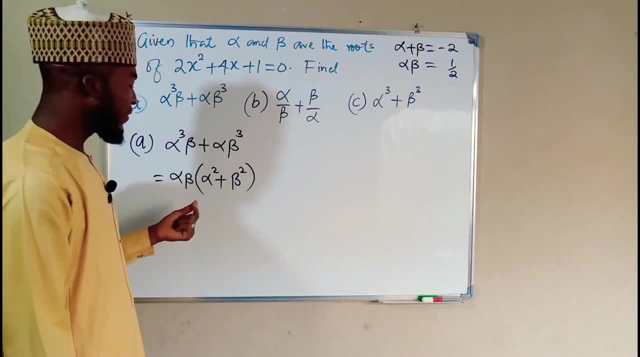 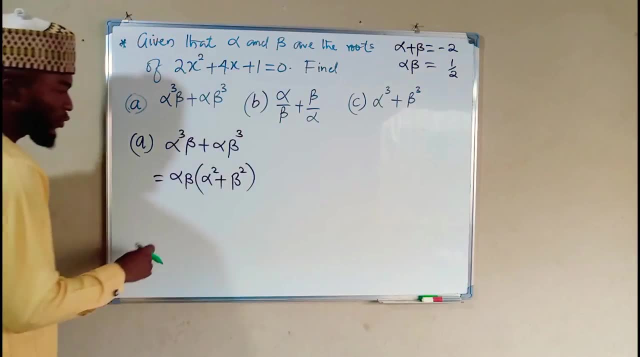 But in our previous lesson you have seen that we have driven this to be equal to alpha plus beta squared minus 2alpha beta. so we can substitute that with the whole product. So we cal enter of the previous definition here that with this this is equal to alpha beta times alpha plus beta squared minus. 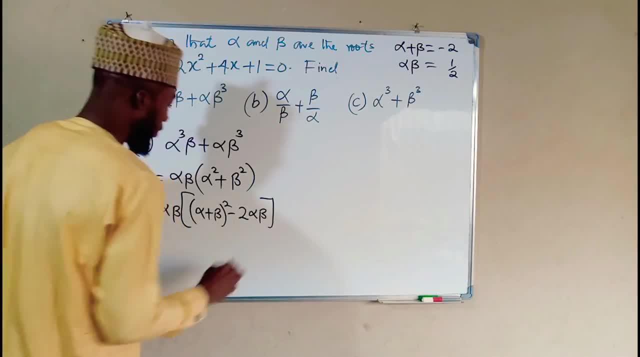 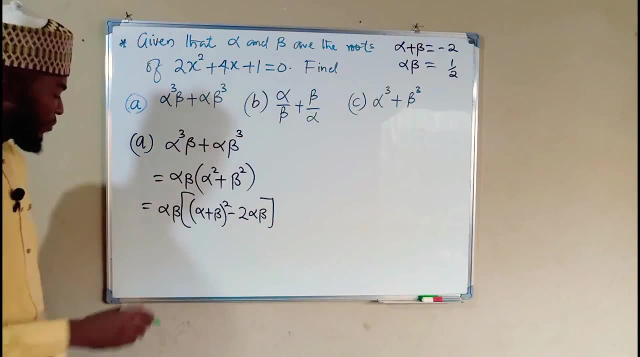 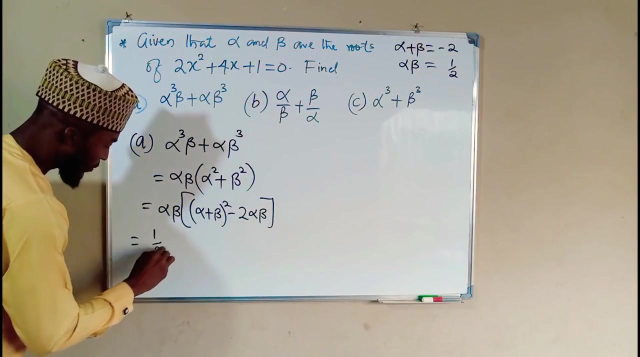 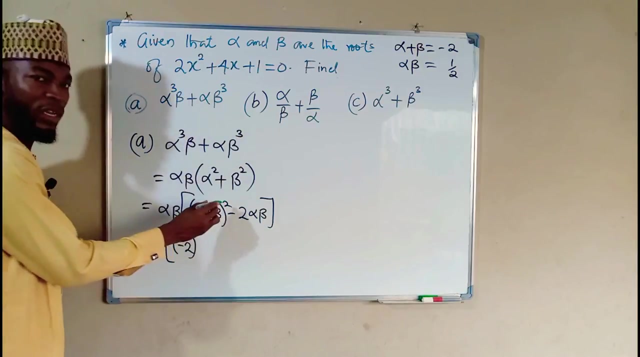 2, alpha, beta, and this is the transformation of this function and we can now substitute our information in here. this is equal to the first. one is product. we have our product to be equal to 1 over 2 times. inside we have the sum which is negative 2. negative 2, but this one contain a square minus 2. then 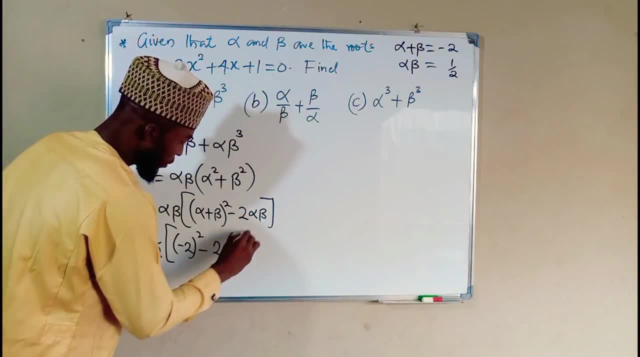 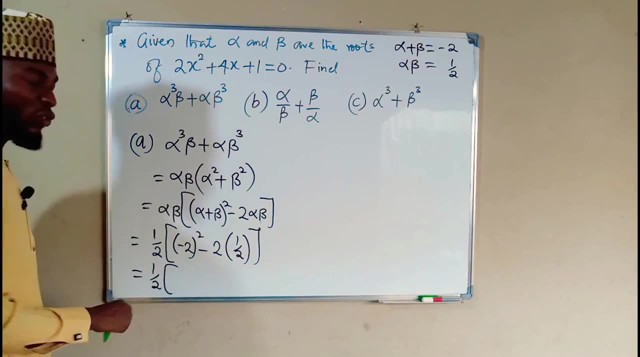 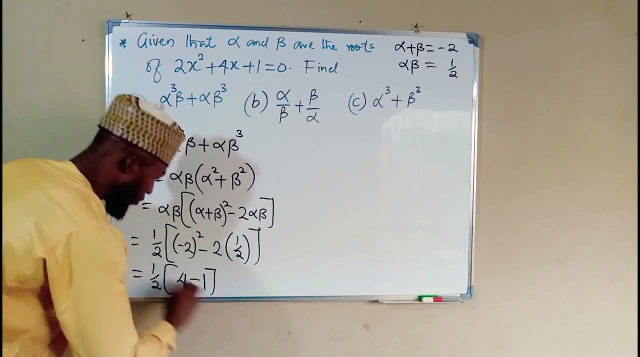 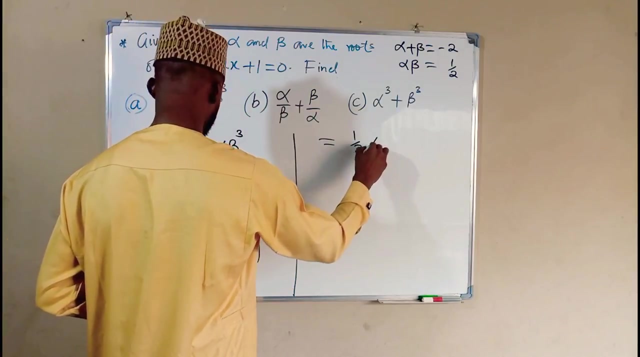 the product is 1 over 2. then we simplify: this is equal to 1 over 2 times negative, 2 squared is 4 minus 2 times a half times negative. 2 squared is 4 minus 2 times a half is 1. so we can say this is equal to 1 over 2 times 4 minus 1 is 3, which is: 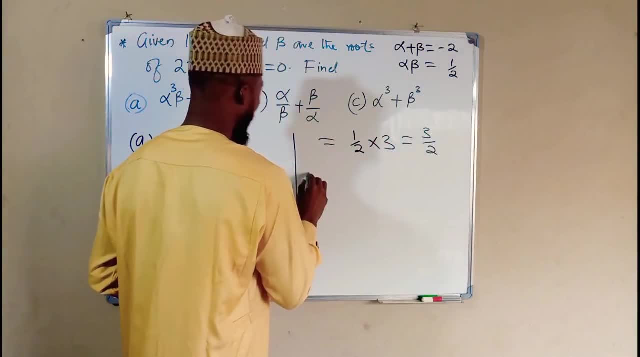 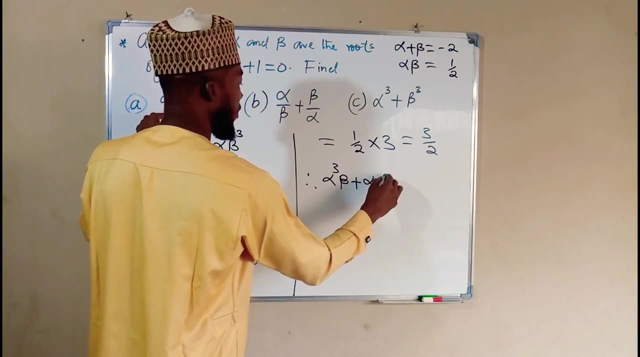 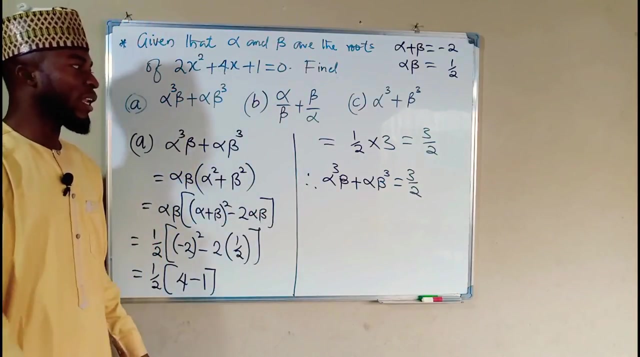 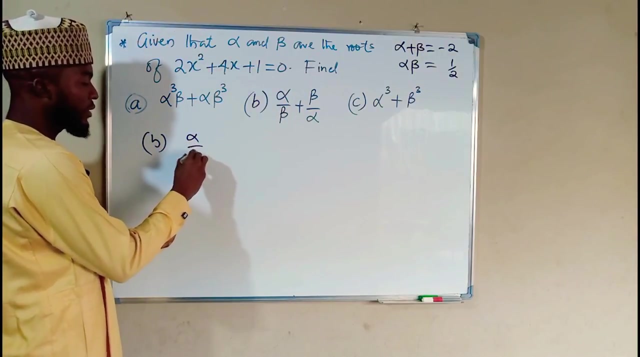 equal to 3 over 2. therefore, alpha cubed, beta plus alpha beta cubed, is equal to 3 over 2, and this is the solution for this first problem. now let us look on to the second one, the second problem. we have alpha over beta plus beta over alpha. again, this does not correspond to any. 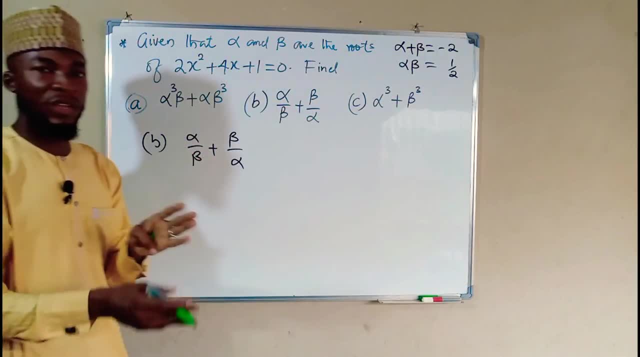 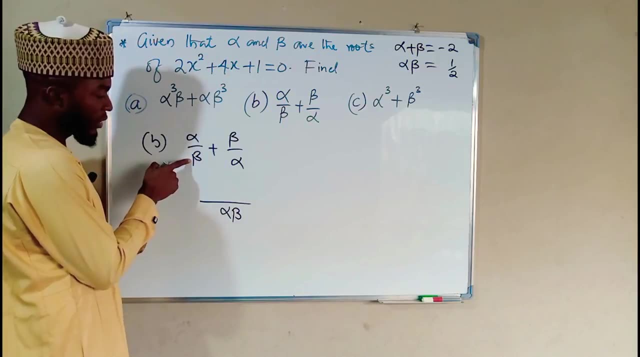 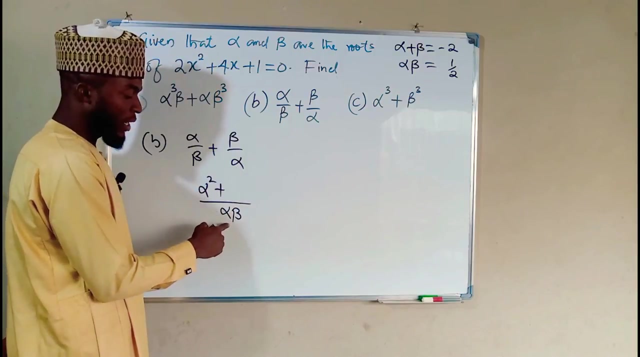 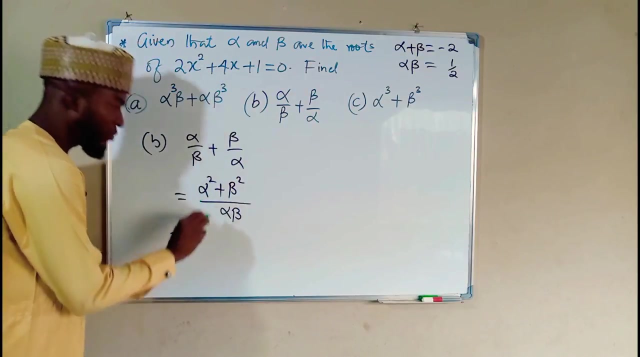 one of this. so let us transform these two units of fractions into a single one, and the LCM is going to be alpha beta. if you plug in beta here, you're going to obtain alpha times. alpha is alpha squared plus. if you plug in alpha here, you're going to obtain beta times. beta is beta squared- alpha squared beta. 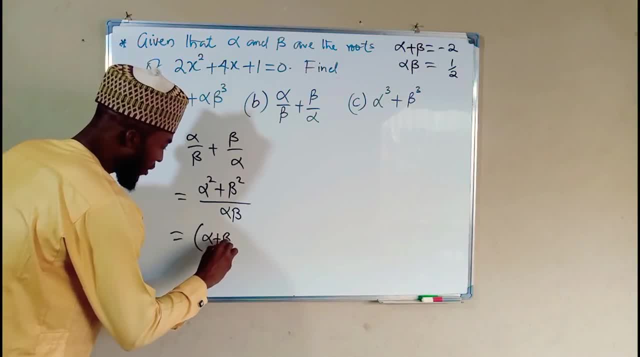 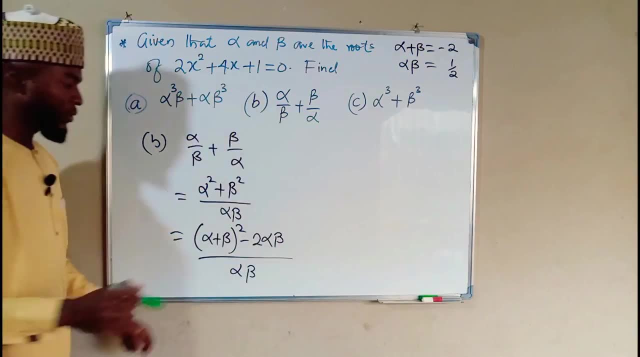 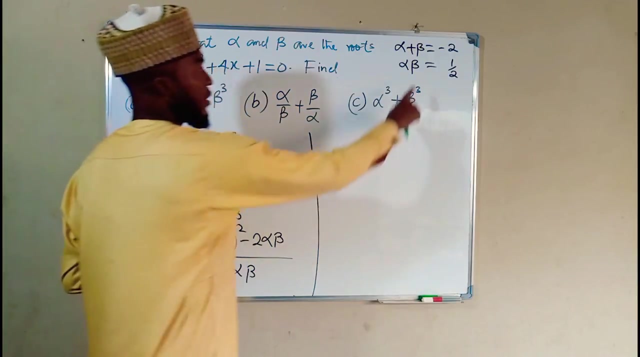 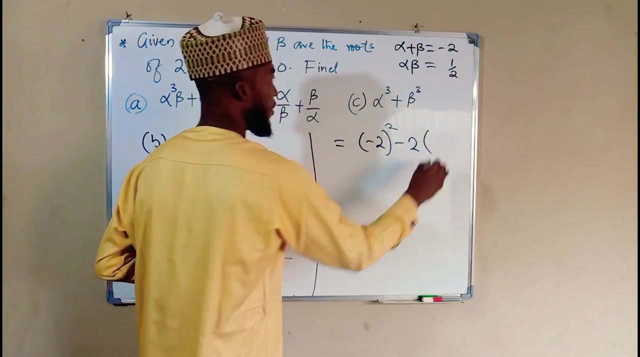 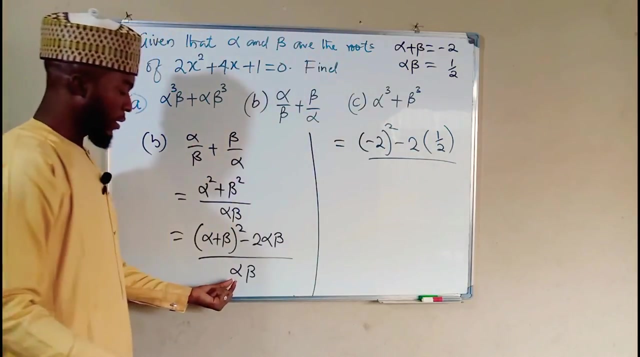 squared is the same thing as alpha plus beta squared minus 2 alpha beta divided by alpha beta. so now let us substitute everything here. the first one we have: alpha plus beta is negative 2, all squared the minus 2 times alpha times beta is 1 over 2, so we have 1 over 2 here. divided by alpha times, beta is 1 over 2. 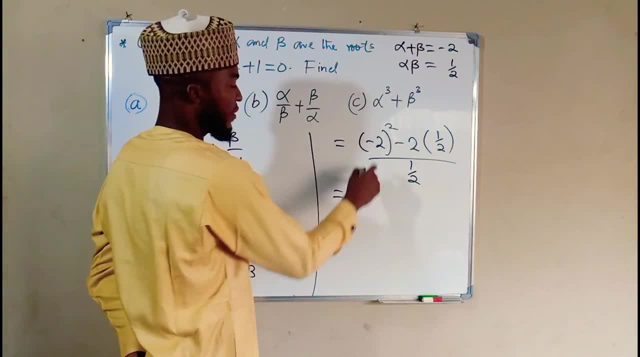 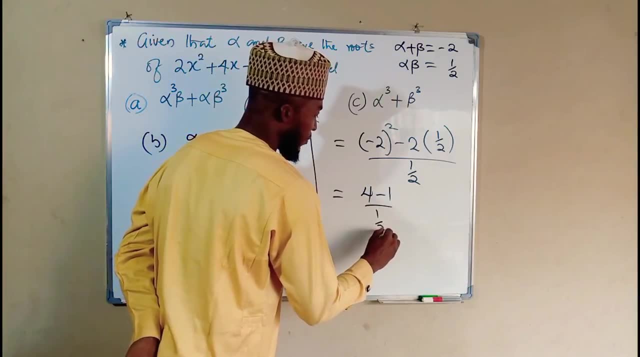 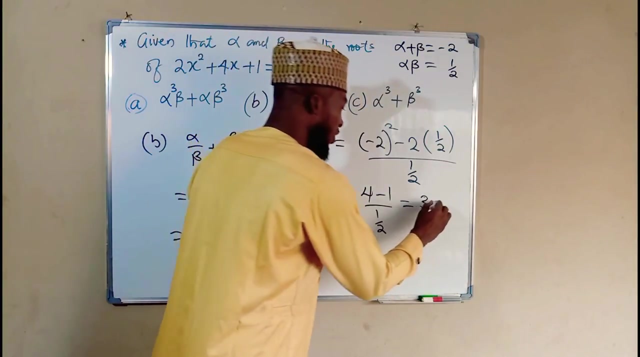 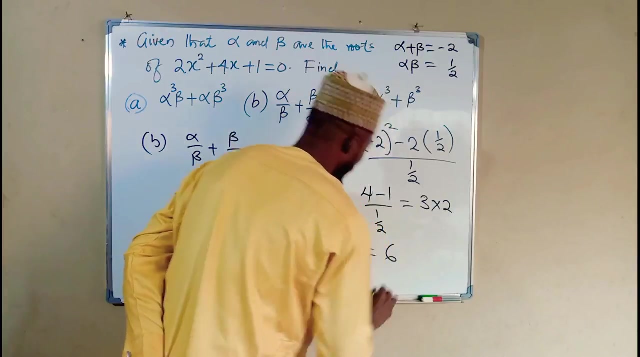 this is equal to. this is 4 minus. this is 1 over 1 over 2. 4 minus 1 is equal to 3. divided by a half is just like multiplying by 2, if you take the reciprocal of 1 over 2, and hence this is equal to 6, which is alpha. 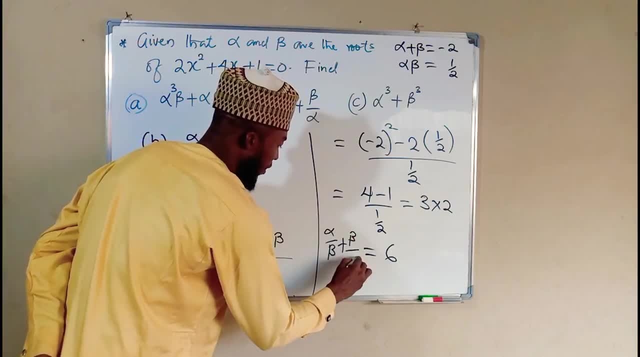 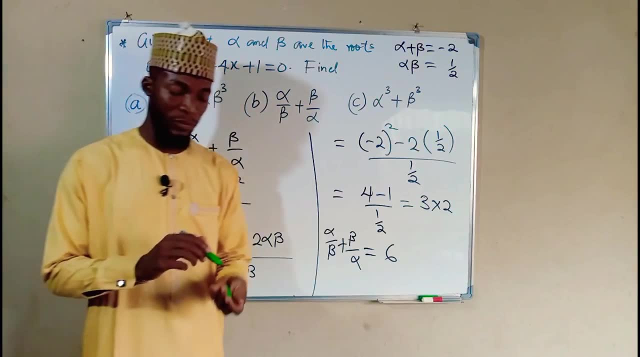 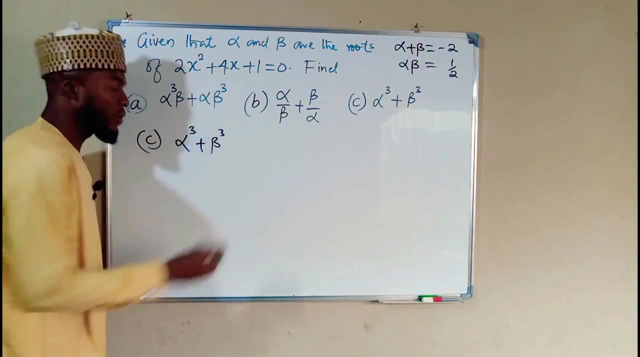 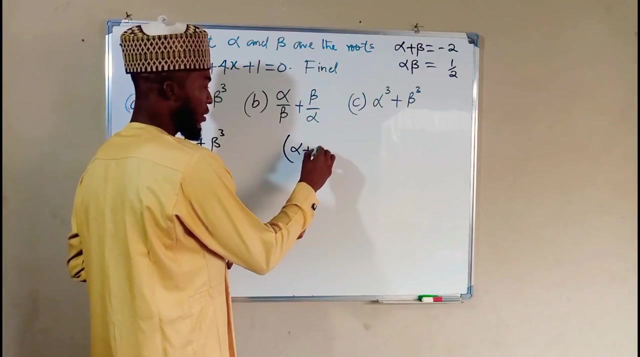 over beta, plus beta over alpha. now let us look on to the last problem which we have as alpha cubed plus beta cubed plus beta cubed. we do not have anything in this form, but once we expand alpha plus beta cubed we shall obtain two times that correspond to this once. so 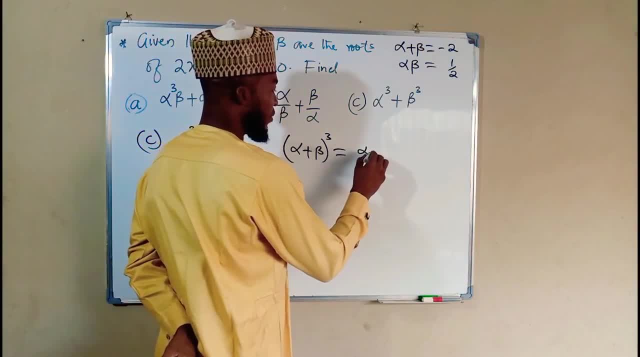 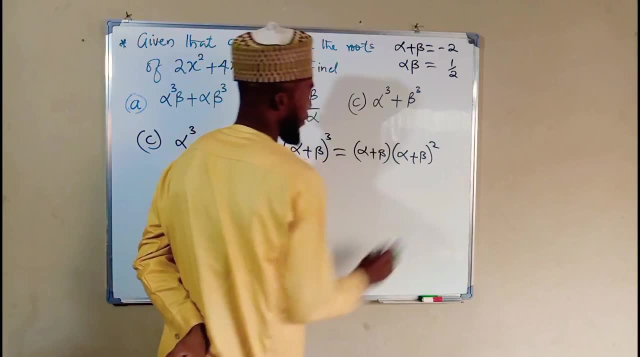 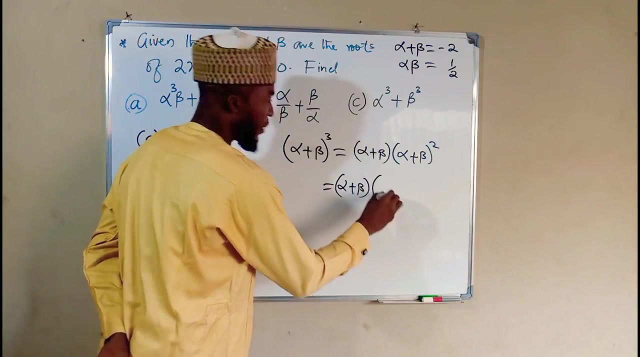 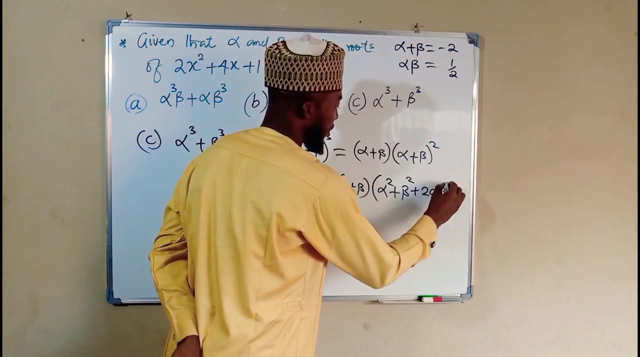 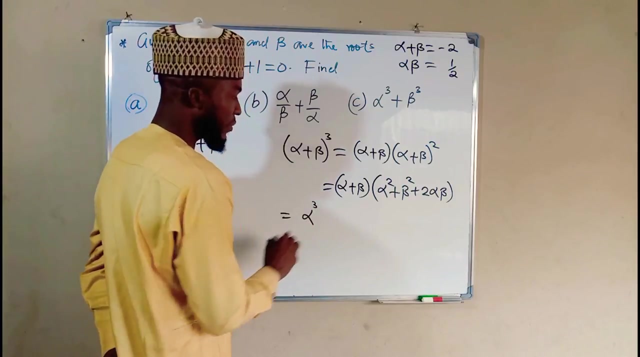 now let us expand this. remember this can be written as alpha plus beta times, alpha plus beta squared. for the expansion of this, we have: alpha plus beta multiplied by the first time, squared is alpha squared plus beta. squared plus 2: alpha beta, now alpha times. alpha squared is alpha cubed alpha. 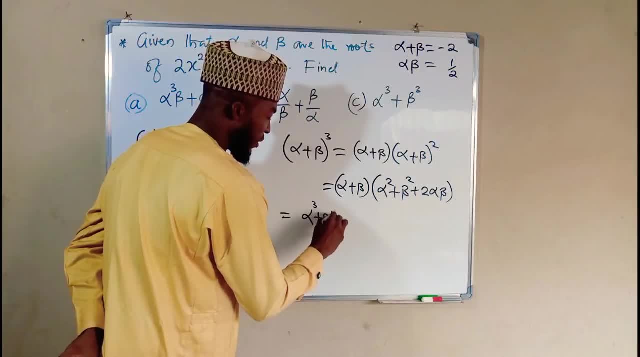 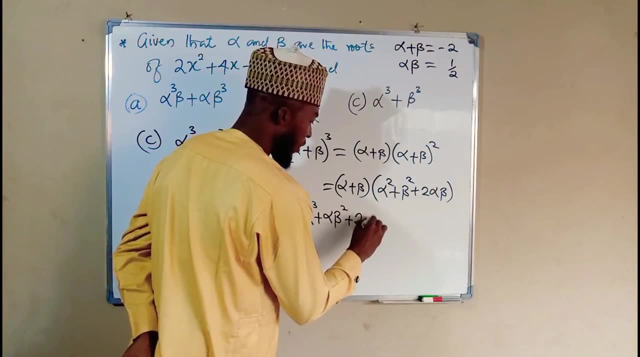 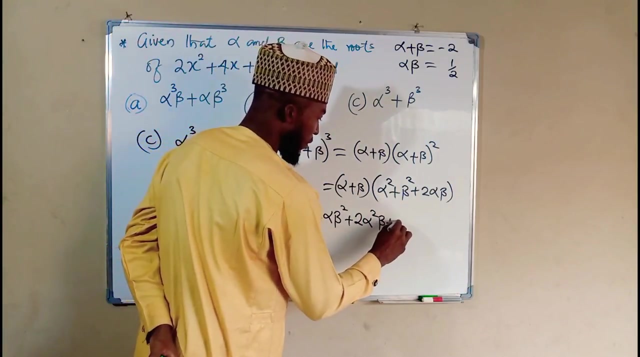 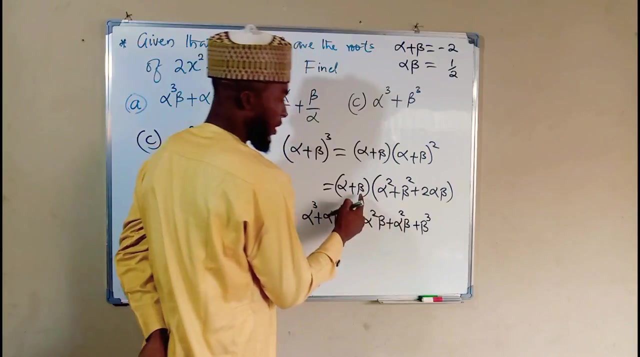 times beta squared is going to be alpha beta squared, then alpha times 2 alpha beta is going to be 2 alpha squared beta. now we move to the second term. this time this is going to be alpha squared beta. this time this is going to be beta cubed, and the last one this time this: 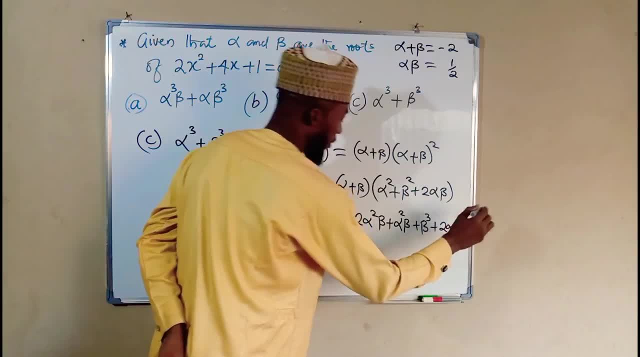 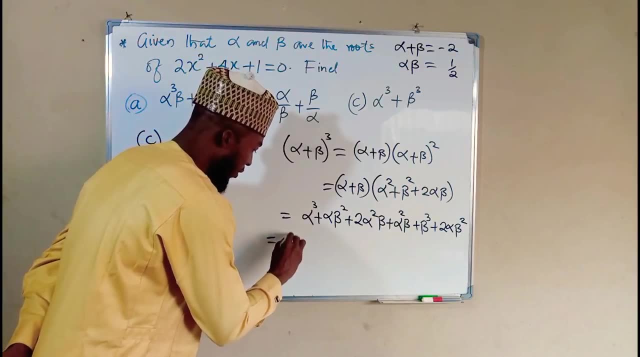 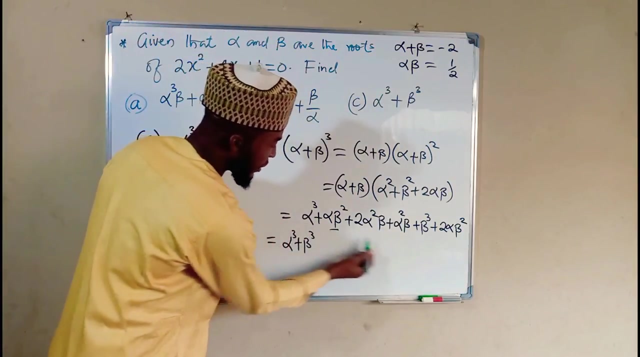 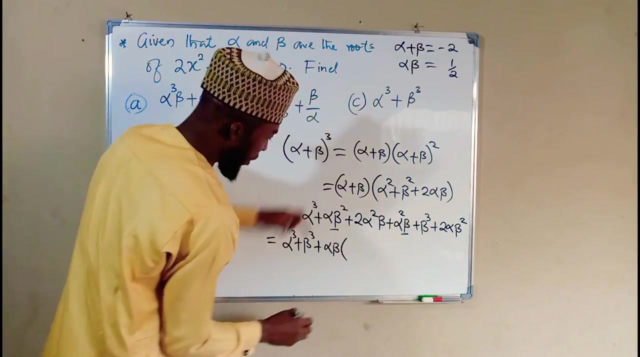 is going to be 2 alpha, beta squared. you can see we have alpha cubed, beta cubed, so we can bring them together, alpha cubed, beta cubed. then we can join these two times together and we can factor alpha beta. so, plus alpha beta, here we will have beta left and here we have alpha left, so we 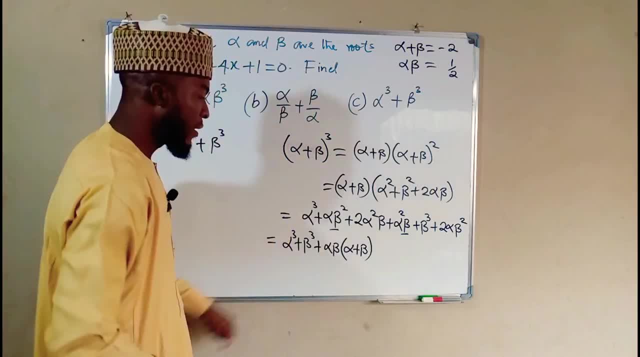 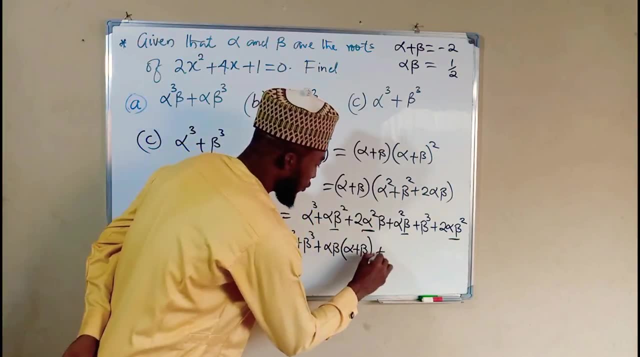 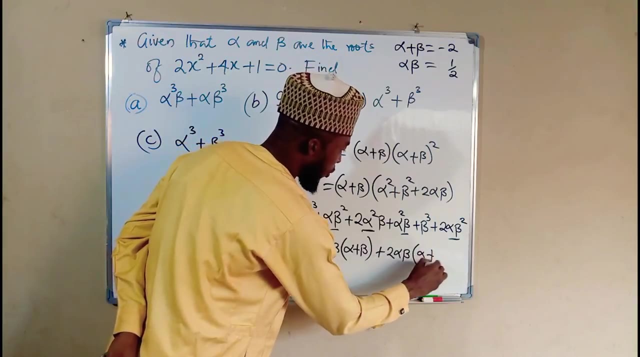 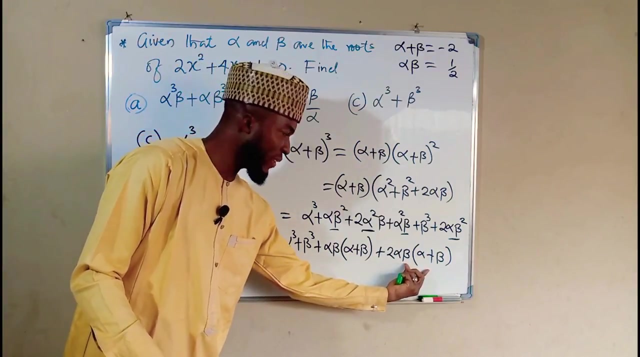 can write them as alpha plus beta and again we can join this two. we can join this and this together, two alpha beta, then inside we have alpha plus, here we have beta, but these two times are the same. we have two quantities of this and we have a single quantity of this if you join them together. 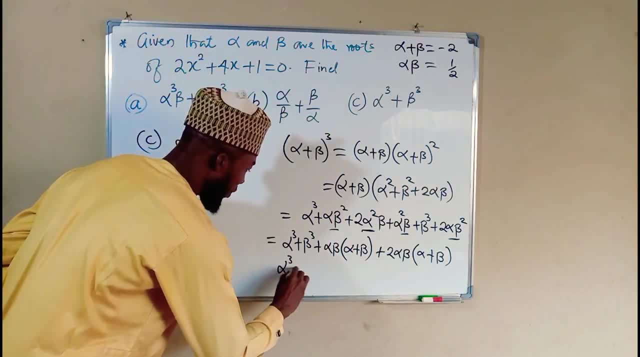 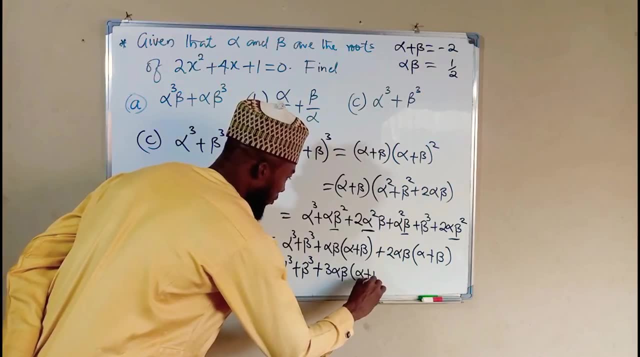 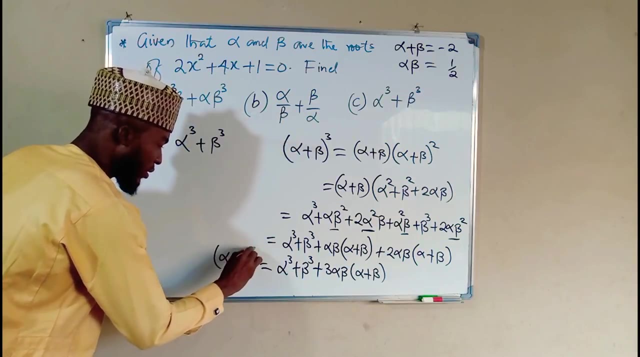 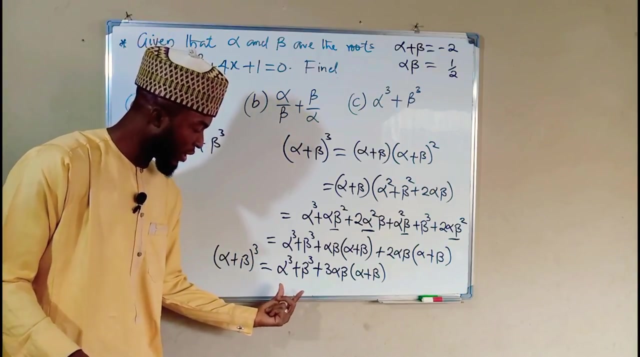 we have three quantities, so we have alpha cubed plus beta cubed, plus three alpha beta times alpha, and all of this equal to the expansion which we have here as alpha plus beta cubed. now, this is what we are looking for, which we can make the subject of this equation by saying this is equal. 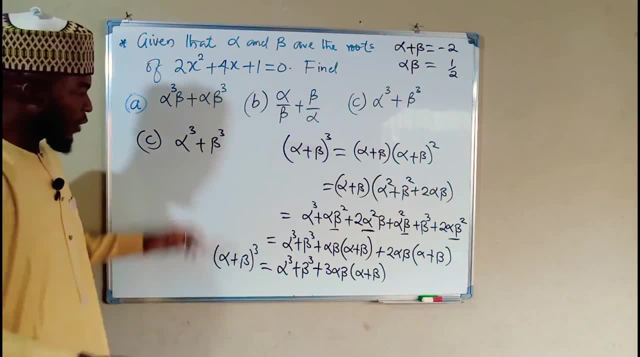 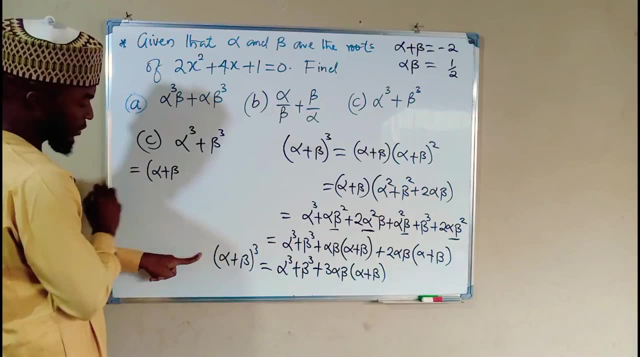 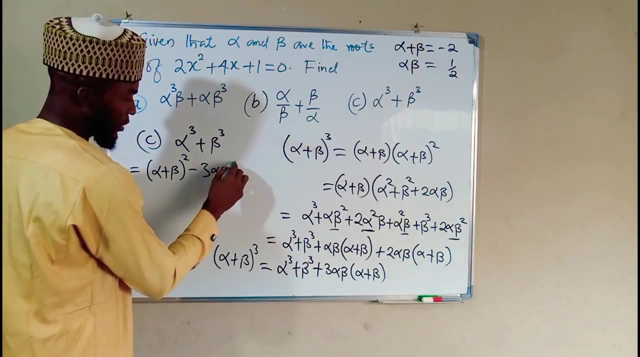 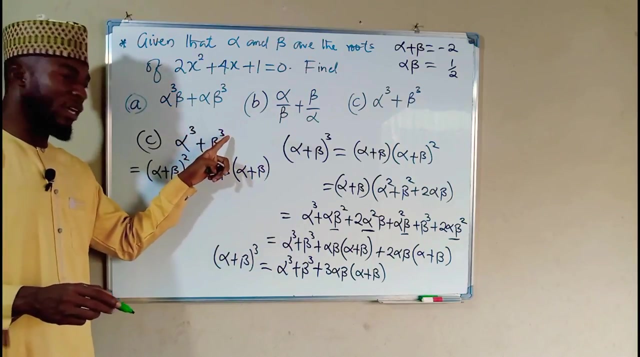 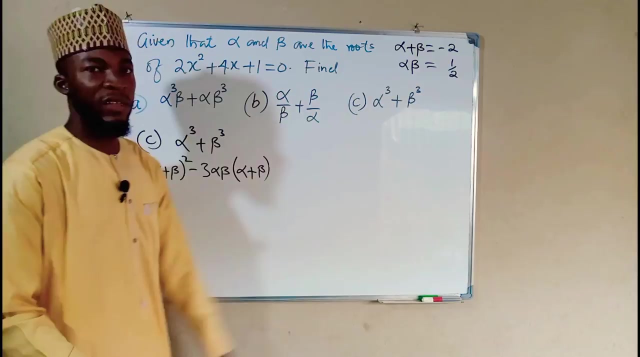 to this, minus this- now we can write it here- this is equal to alpha plus beta cubed. then minus three alpha beta times alpha plus beta, this is what we have as alpha cubed plus beta cubed. now let us substitute everything here. alpha plus beta is given as negative two, so we have negative two. 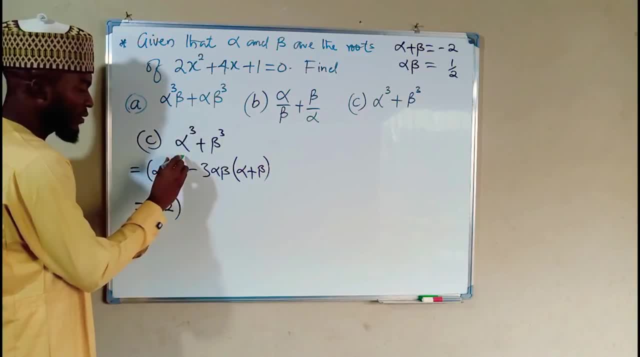 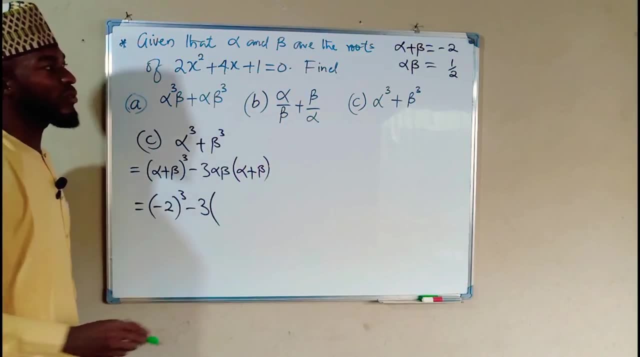 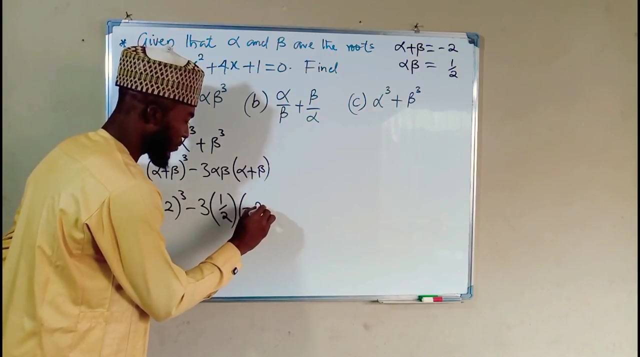 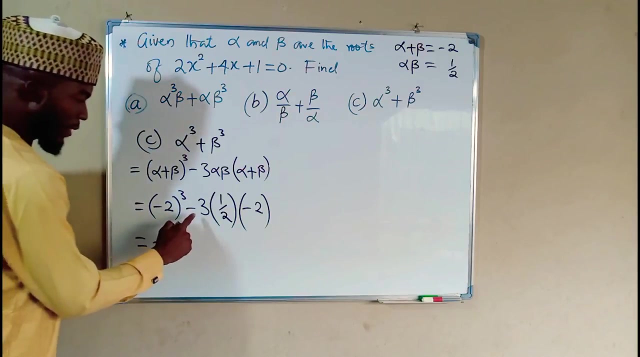 but this is not a square but a cube. sorry for that, this is a cubed. the minus three times alpha times beta is one over two. then multiply by alpha plus beta, which is negative two. this is equal to negative eight. because of this multiplication, this will transform this to positive. 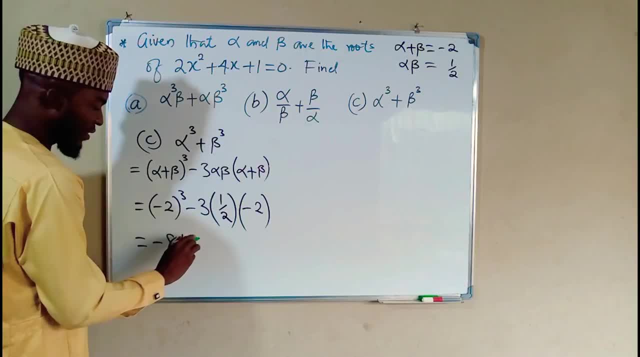 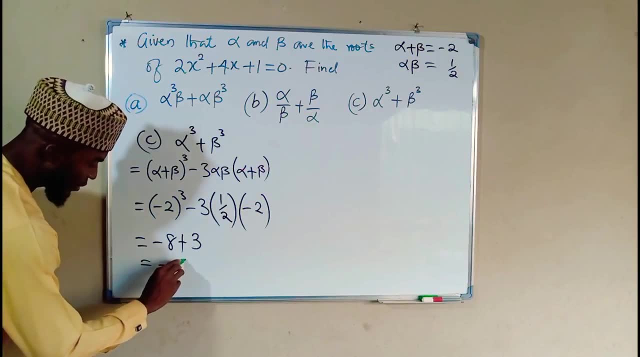 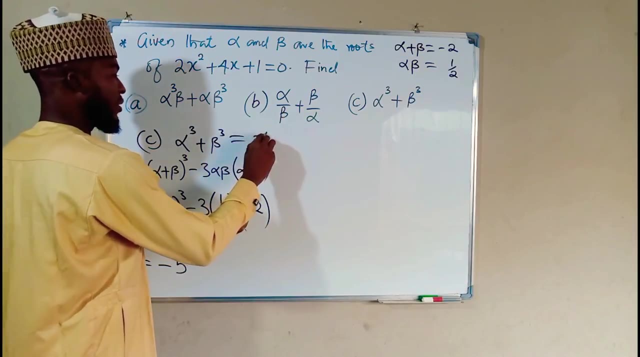 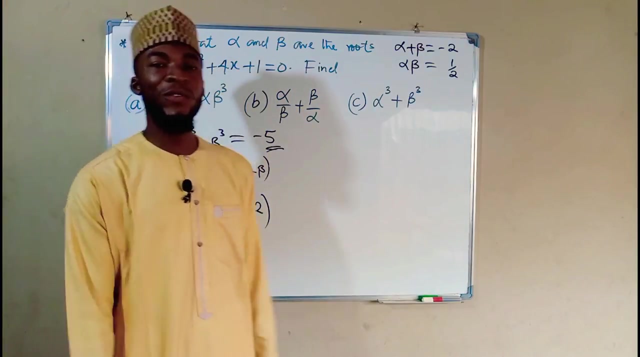 this time, this is one time, this is three, this is equal to negative five, which is just equal to alpha cubed plus beta cubed, and hence this is the solution for this problem, and this is all I have for you today. thank you for watching and do have a nice day.